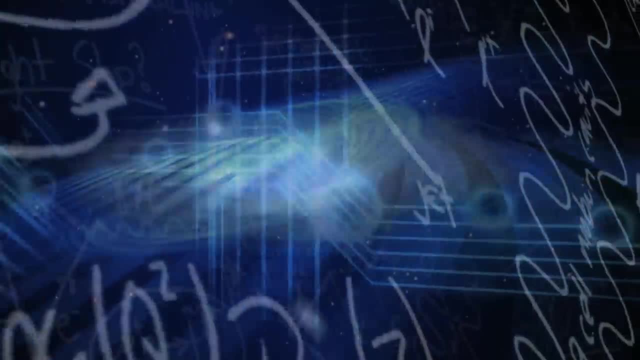 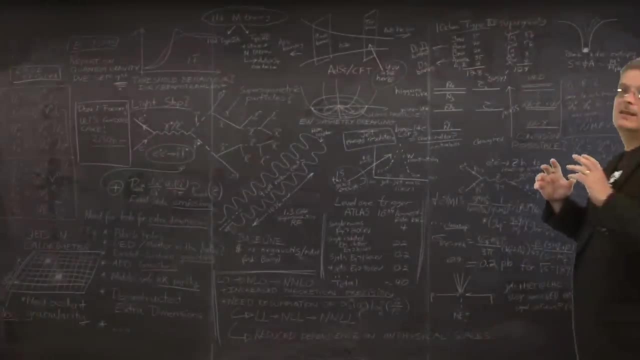 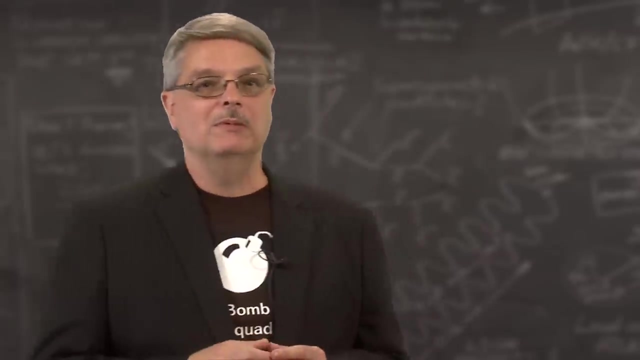 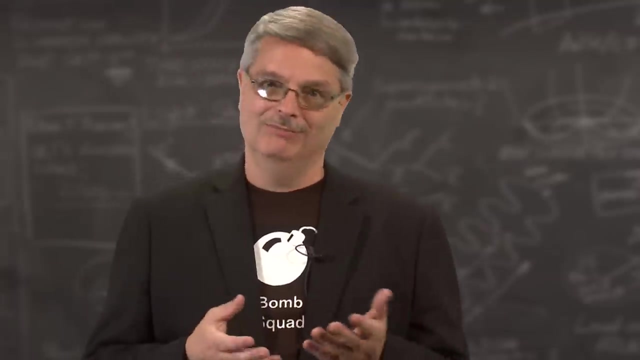 You've probably seen a few of my videos by now, so this makes us old friends. You've also probably deduced that I'm not always an urbane and charming video host. In fact, during the day I'm a physicist. Well, still urbane and charming, to be sure, but a physicist. 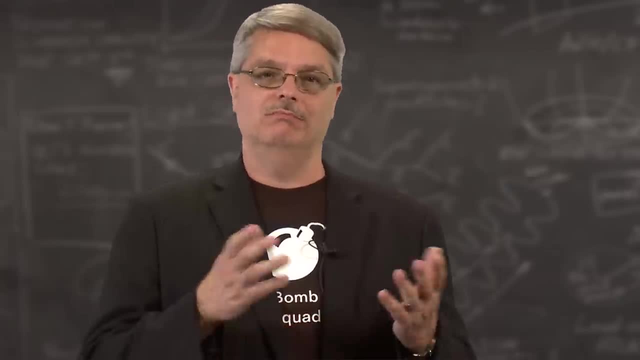 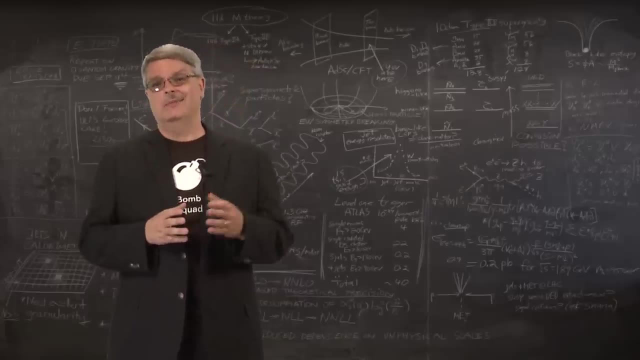 And to be more specific, I'm an experimental particle physicist, which is the most awesome kind of scientist to be. So how does a particle physicist make a measurement? Well, in my case, I take two particle beams and smash them together like two cars in a head-on collision. 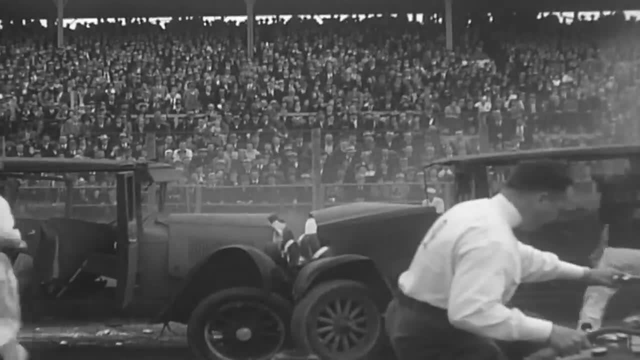 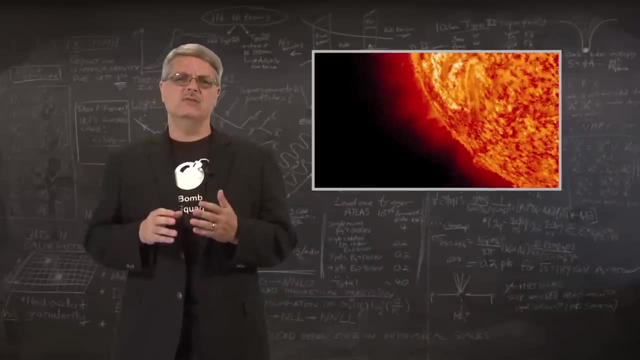 In these collisions, we can heat matter to incredible temperatures, as much as 100,000 times hotter than the center of the sun. This allows me to study the conditions of the universe about a trillionth of a second after the Big Bang. The fact that we can do this continues to amaze me. 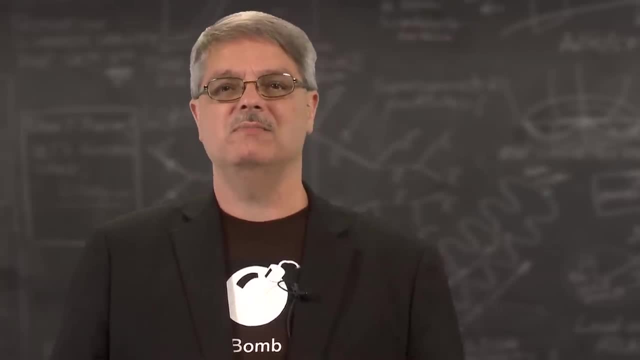 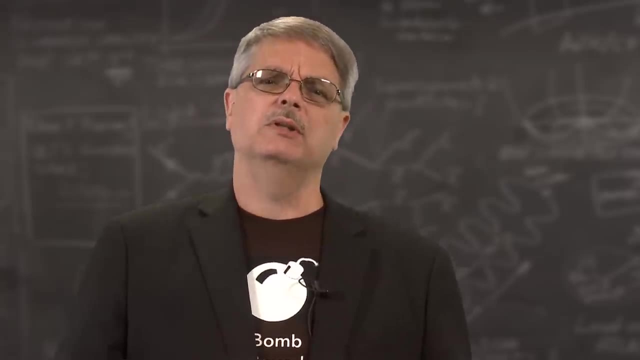 I mean, if the fact that mankind has developed this kind of power doesn't make you at least a little proud of your humanity, well, I don't know what will. So how is it that we are able to understand matter under these extreme conditions? 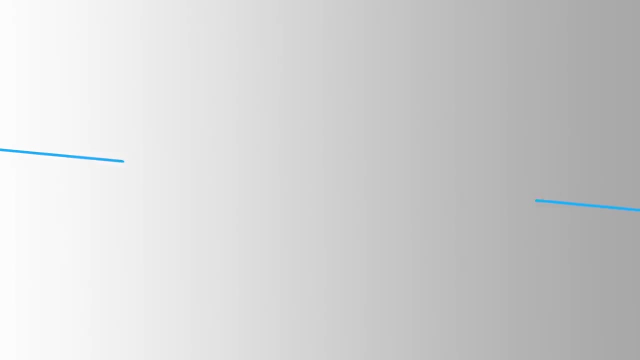 You've no doubt seen animations like these. Two beam particles come together and collide. After the collision, hundreds of particles can come out of it. The actual collision takes the unimaginably short time of under 10 to the minus 23 seconds, Even the relatively long time that the collision persists in our detector. 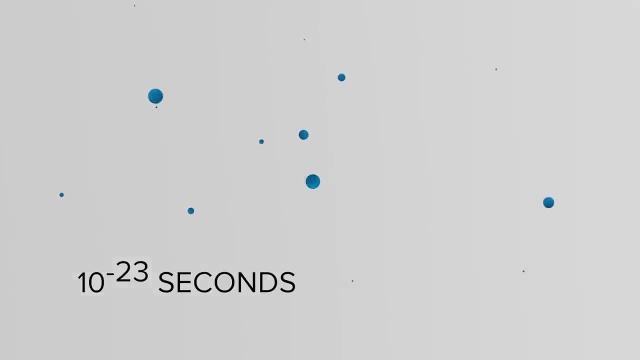 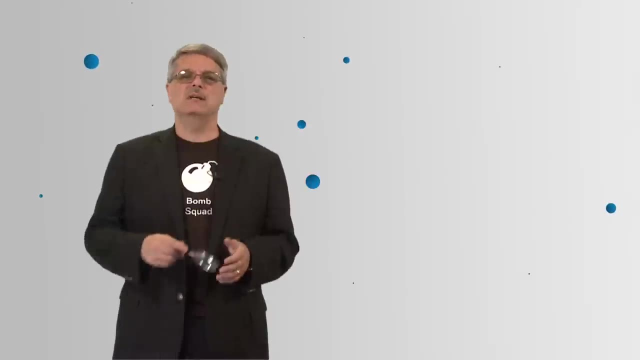 is still incredibly short, say in the ballpark of a couple billionths of a second or so. So how is it that we are able to make measurements of particles coming out of the collisions? I mean, it's not like we can watch the particles themselves. 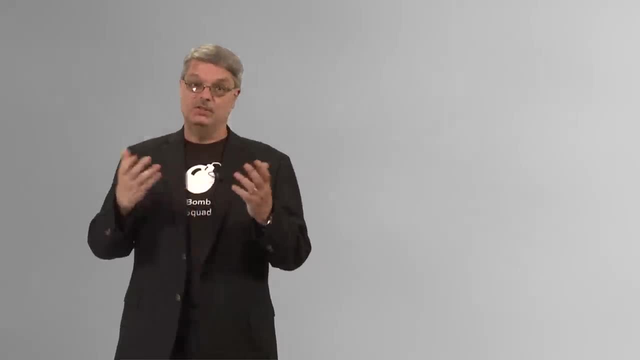 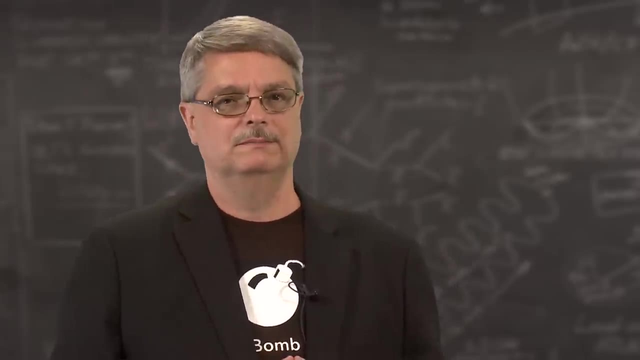 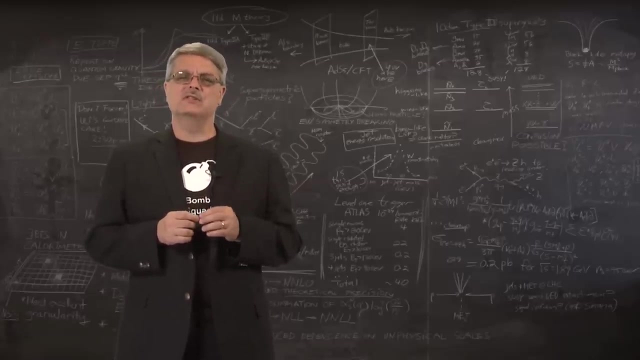 Unless they are interacting somehow with our detector, they are just simply invisible. Yet scientists study billions of collisions. What's our trick? I can explain this pretty easily by means of an analogy. This might surprise you, but particle physicists employ the same basic techniques. 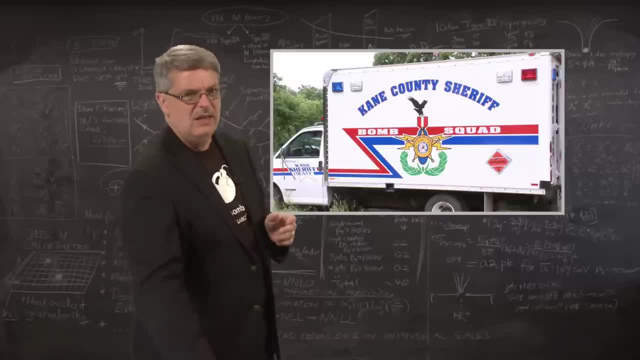 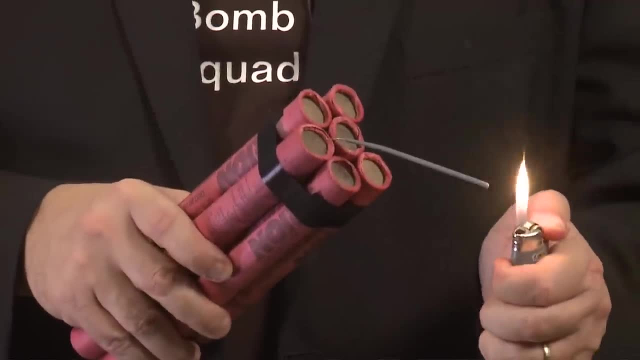 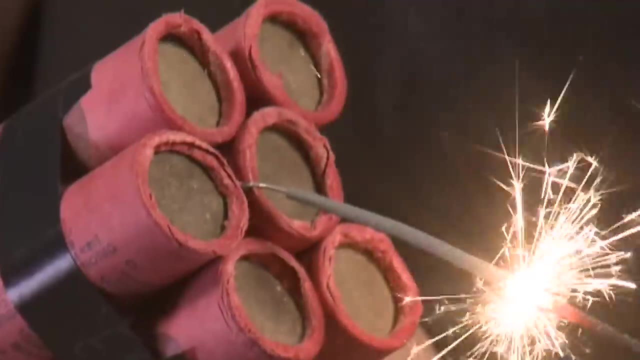 as those used by bomb squad investigators. So how do bomb squad investigators do it? Well, the first thing is they don't stand by the bomb when it goes off. Let's imagine how that would work. Ow Man, I hate it when that happens. 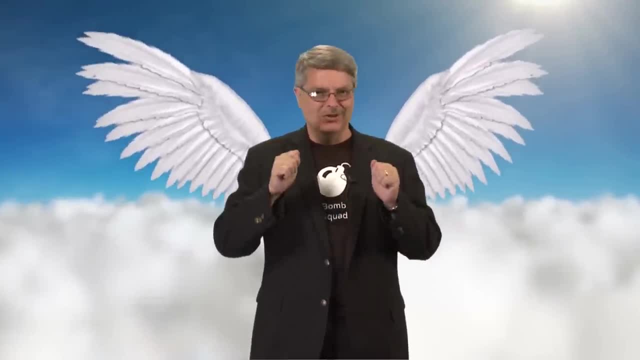 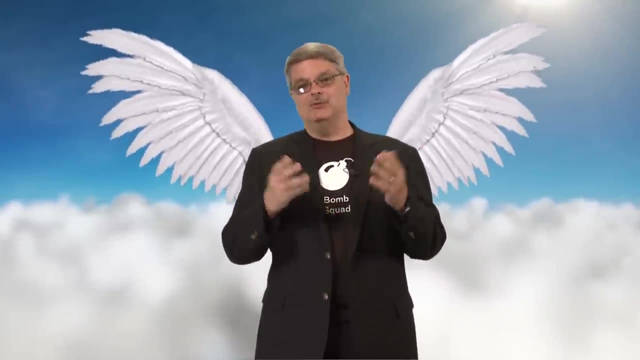 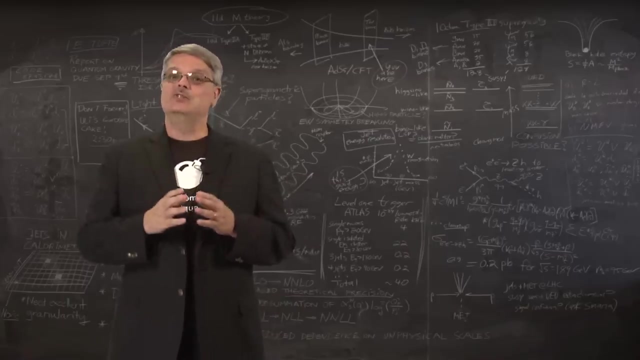 Don't let anyone tell you that you get used to getting blown up. It hurts every time. You can see why this isn't a good way to understand an explosion. Maestro, can you bring me back? That's better. So how do the experts do it? 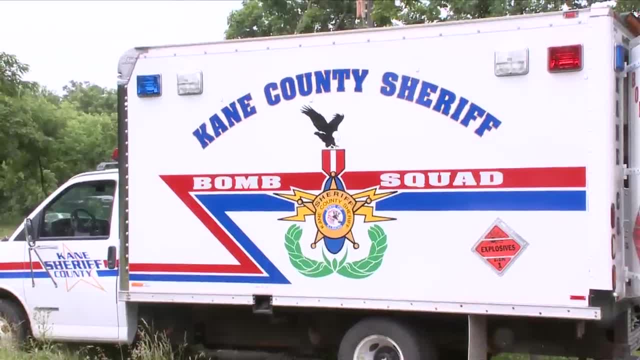 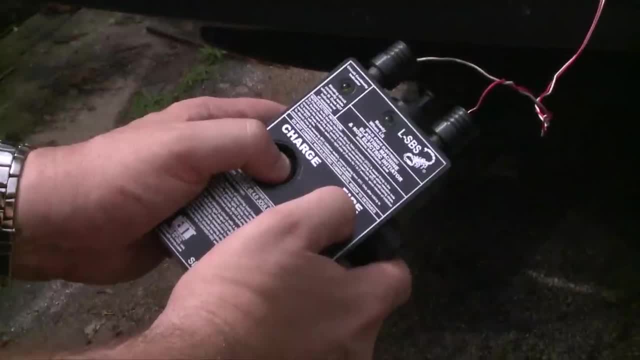 To give you an idea. we asked help from a local bomb squad. We asked them if they could show us how it's done And luckily they allowed us to come along on a training exercise. Now I hope I don't have to tell you guys. 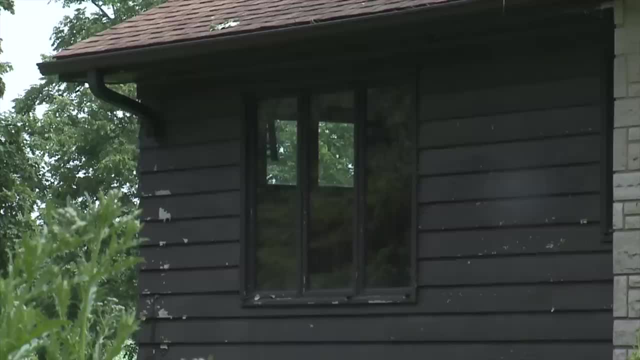 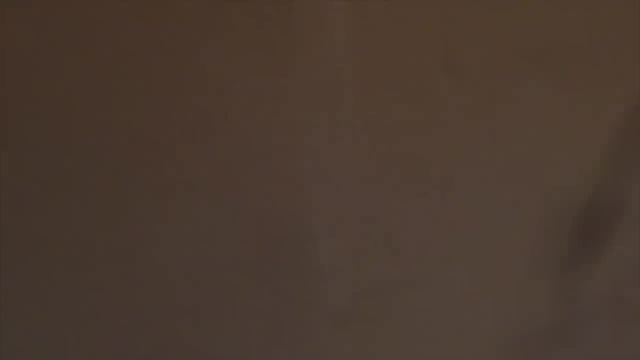 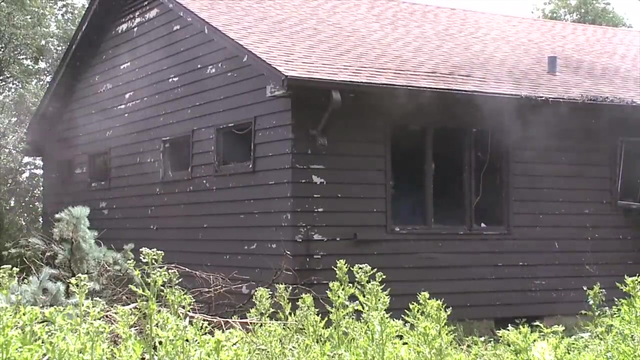 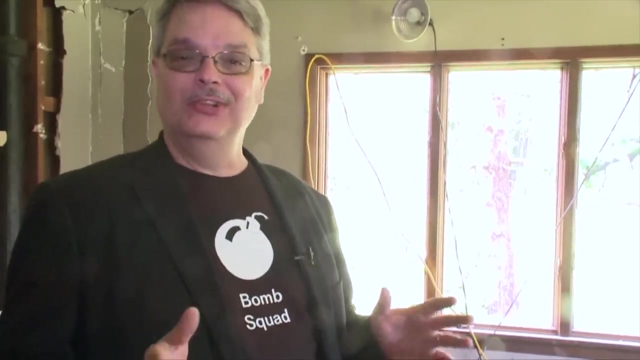 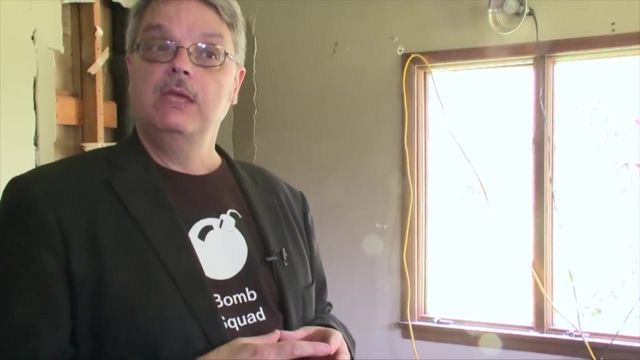 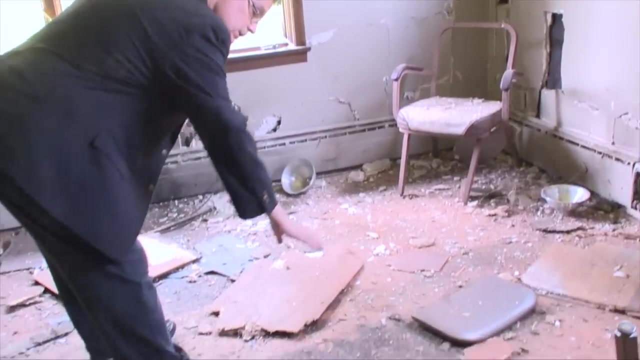 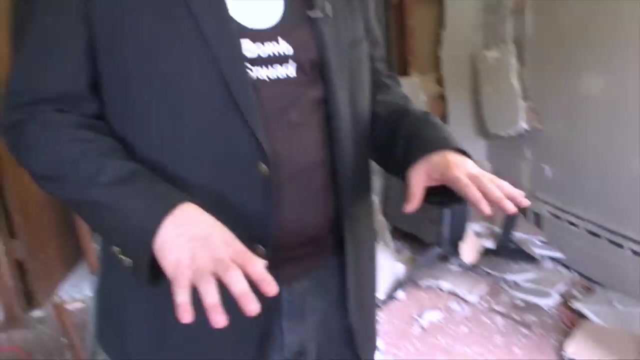 Kids. don't try this at home. Five, four, three, two, one. that simple bit of information. we know that the explosion was in this area. 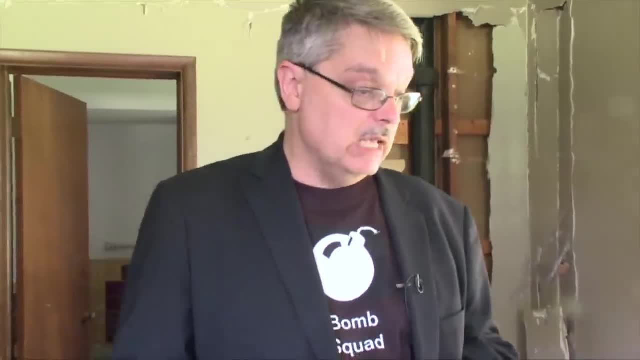 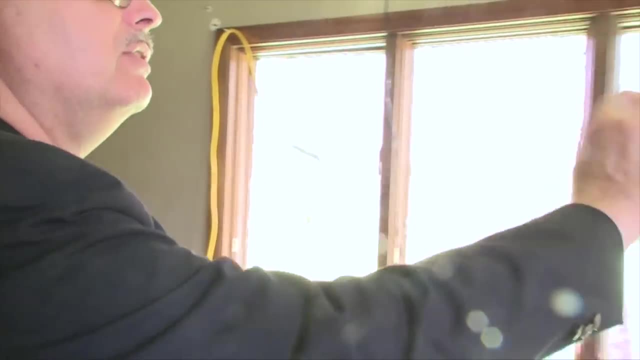 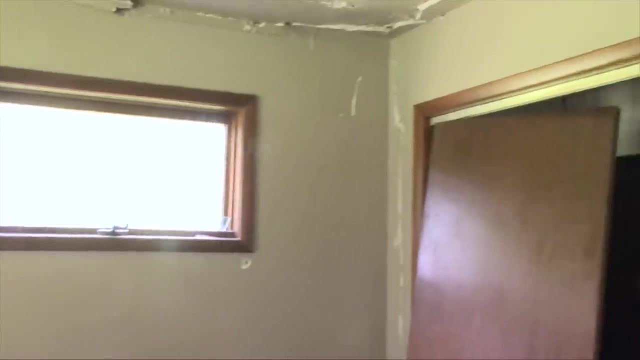 rather than another part of the room. We also can take a look at the corners of the room. here, For instance, we see the corner over here is significantly damaged and in addition this corner here is also completely destroyed. In contrast, the other side of the room, the corners are far less damaged. That information in 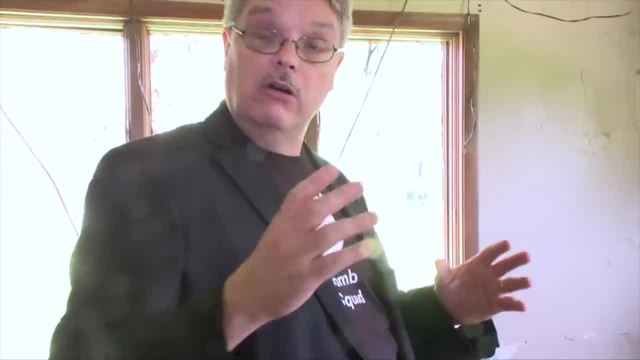 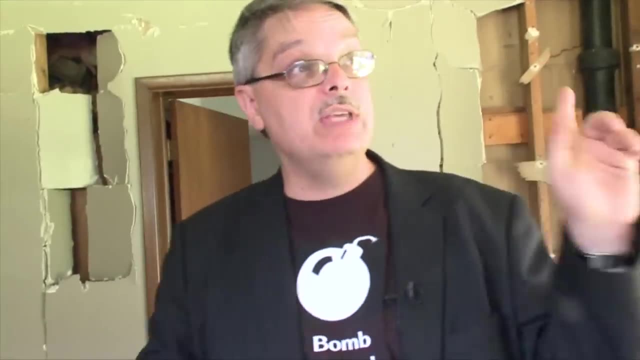 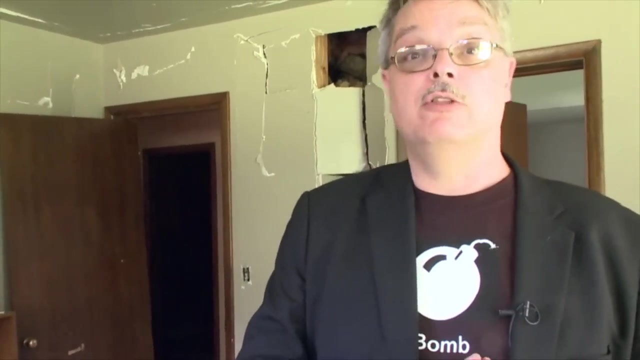 addition, confirms the location of the explosion, because corners focus the, the effect of the explosion, And so both of these messages also confirm the message of the, the blast damage on the floor. The explosion was on this side of the room. In addition, if we look in the ceiling up here, we see several holes in. 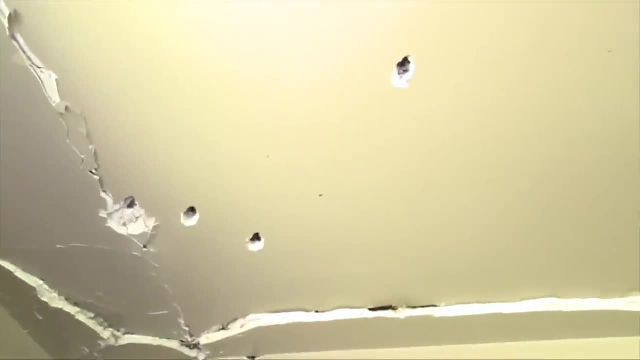 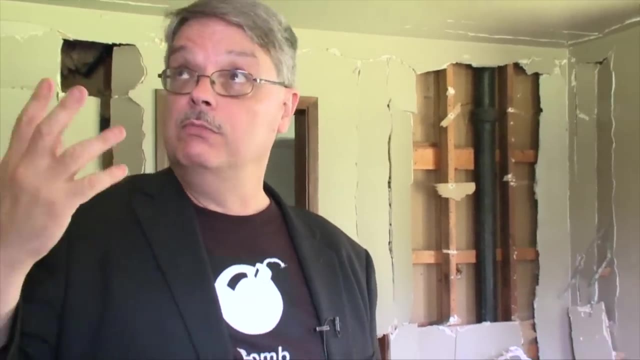 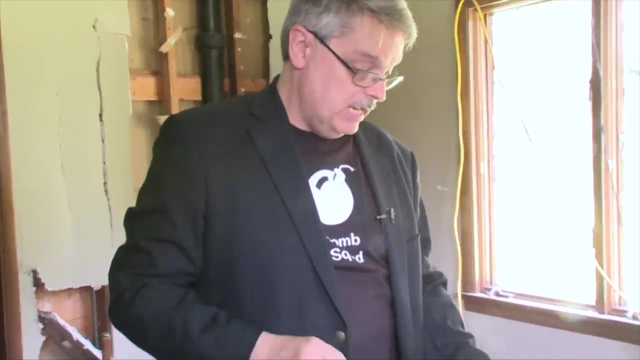 the room and that is shrapnel damage where the bomb punched holes in the ceiling. These could be ball bearings or nuts or something like that, some piece of metal. Now we happen to know exactly what we did: We cast a set of bomb right here in the cabinet, which we see is 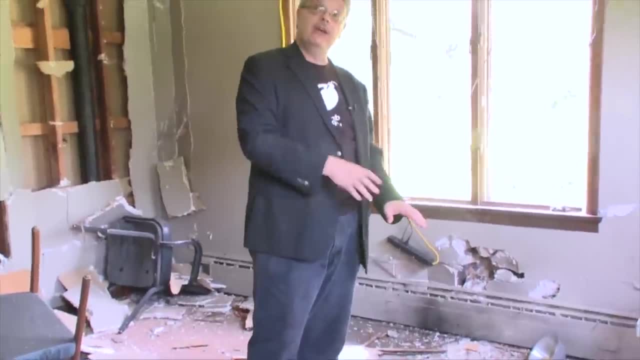 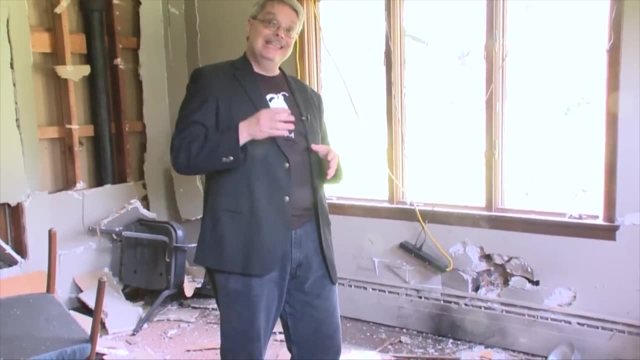 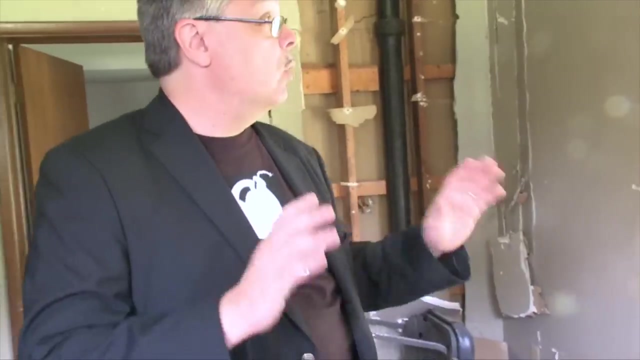 completely destroyed and we put some ball bearings that fired in that direction. So what we know is that the room is confirming what actually occurred, and that is how you do a bomb investigation: You're never there when the explosion occurs. What, instead, is? you ask yourself: what do the surroundings 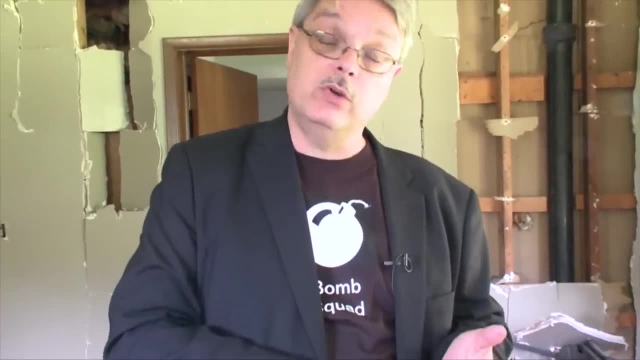 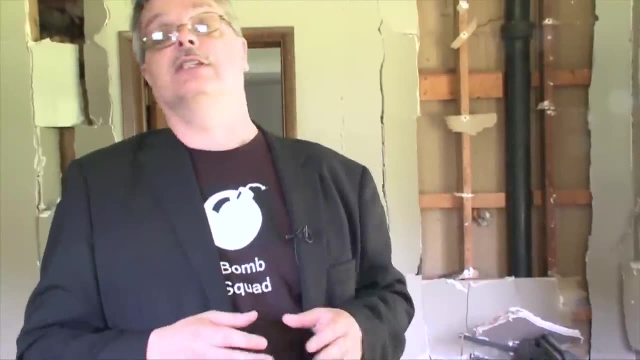 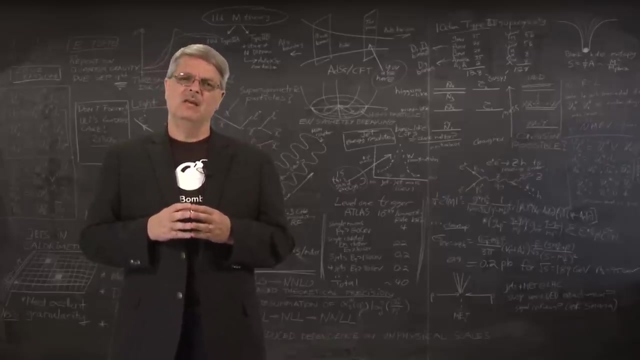 tell us And from that we reconstruct the bomb, the location, the yield and all that information. And that's exactly what we do, or analogous to what we do in particle physics collisions. So how does this relate to detecting particle physics collisions? Well, scientists can't. 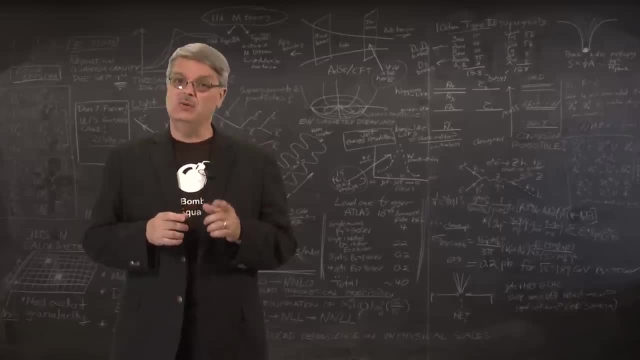 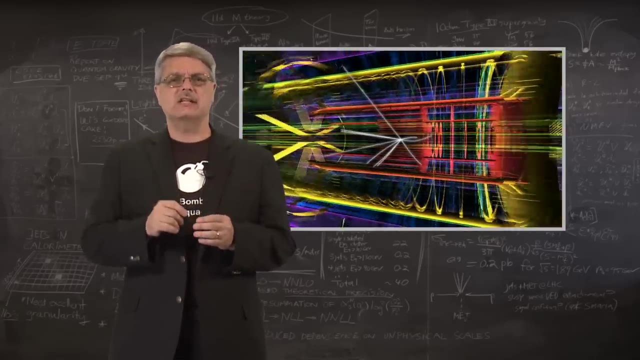 directly study the particles coming out of a collision. so what they do is arrange the collisions to occur inside a detector. And this is the crucial point. It's not just any detector, It's a detector about which they know a great deal. They have carefully. 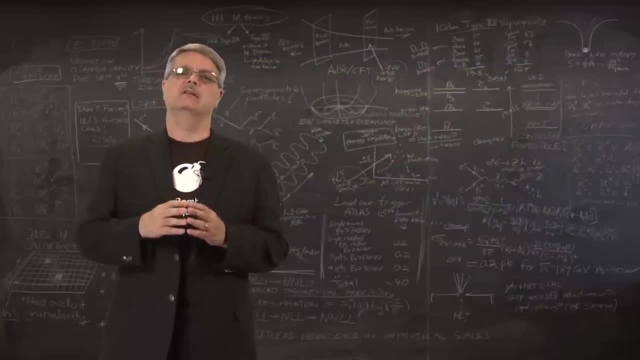 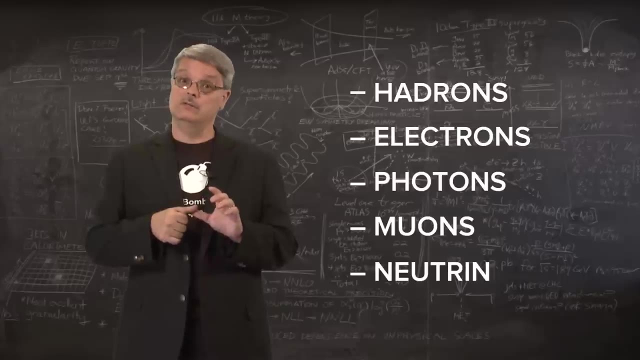 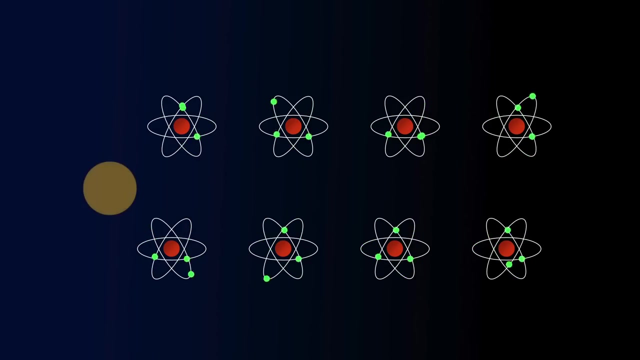 designed it keeping in mind the myriad of particles generated in a collision. These particles have many names, like hadrons, electrons, photons, muons and neutrinos. Each of these interact differently with matter. For instance, electrons, muons and some hadrons have an electrical charge. A particle with 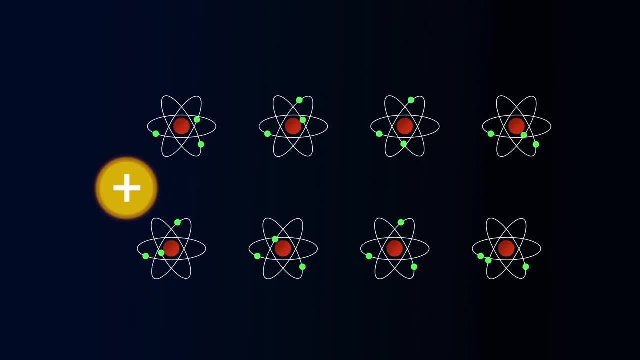 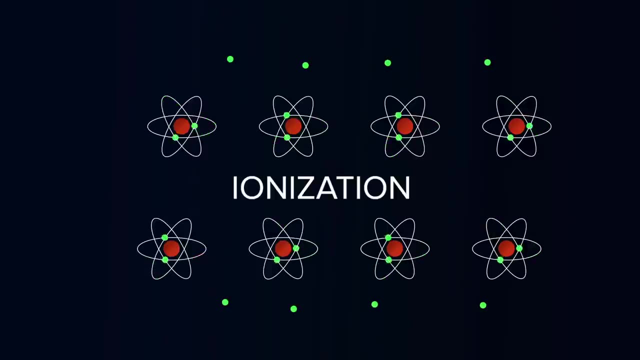 electrical charge generates an electrical field around it that knocks electrons off of atoms as it goes through matter. The technical name for this phenomenon is ionization. The scientists look for the effects of free electrons in their equipment. If they see a string of free electrons, there's. 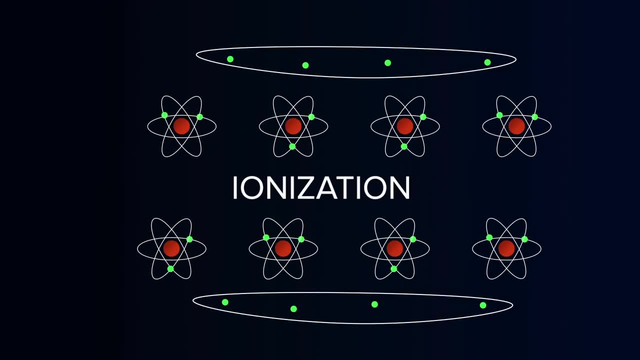 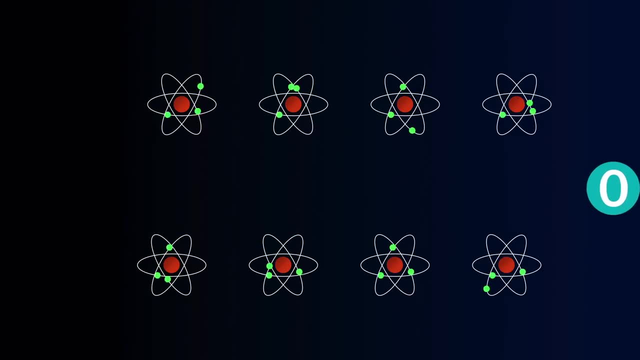 a good chance that an electrically charged particle has passed through their detector. However, photons, neutrinos and some hadrons don't interact in this way and such a detector wouldn't see them. In order to see these unseen particles, we 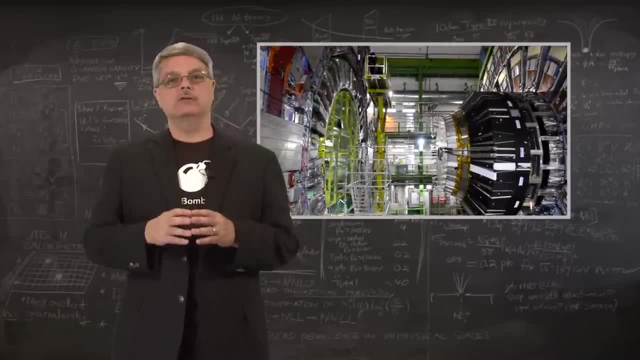 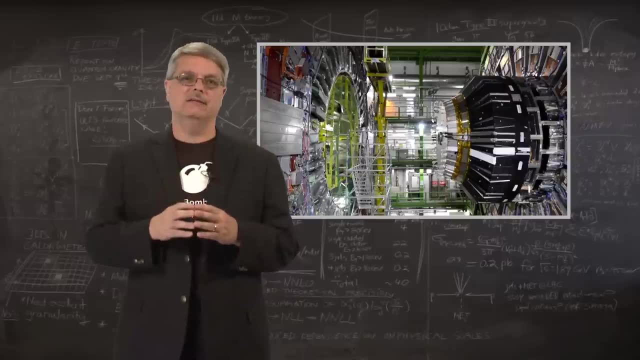 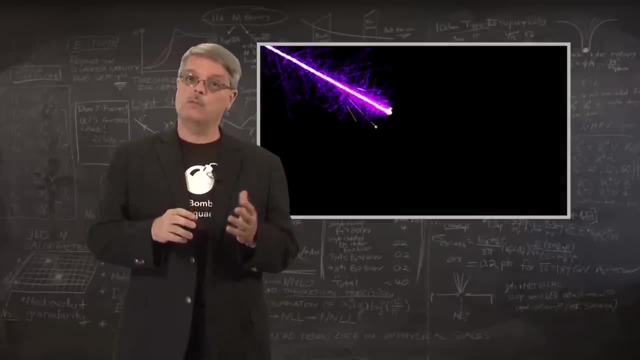 need to add other detectors which react to different ways in which particles interact with matter. For instance, hadrons, electrons and photons smash into atoms and do a most curious thing: They make more particles. For instance, one of these particles hits an atom and two or five or even more particles come out. These new particles. 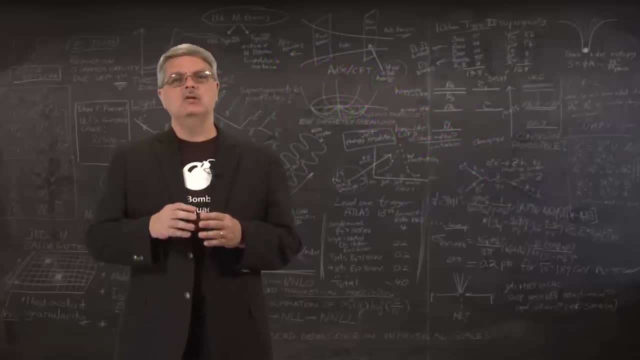 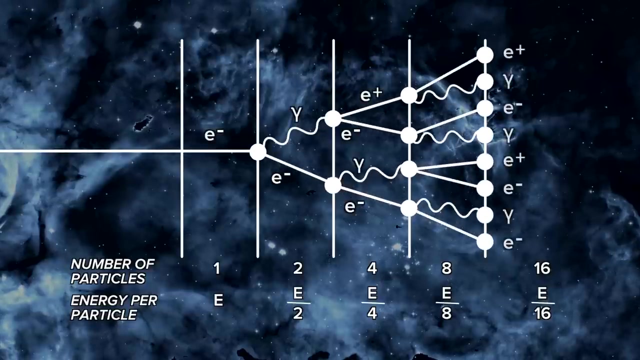 can then interact with more atoms. Using the simple scenario in which a single particle interacting with an atom makes two particles, we can see how a single particle makes many, Starting with a single electron. one particle goes to two, which goes to four, then eight, then sixteen, and so on. 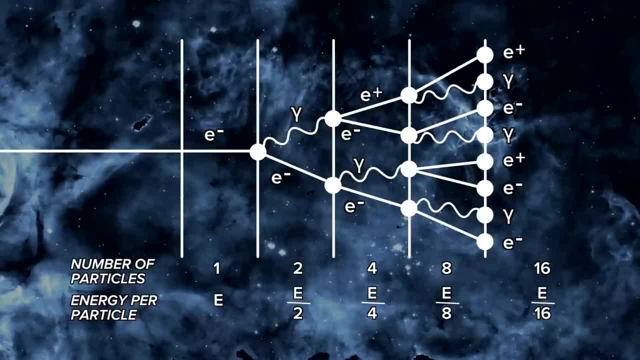 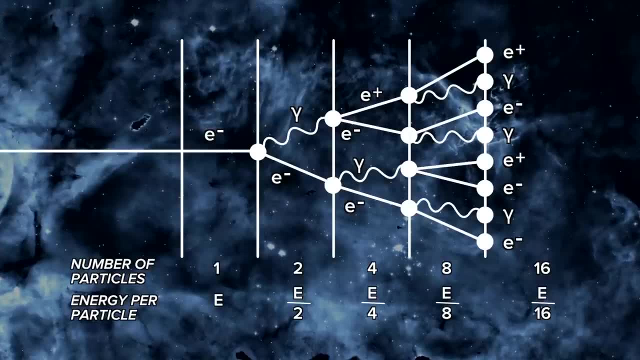 Pretty quickly. a single particle can turn into thousands or tens of thousands, Since energy is conserved. every time new particles are made, they have lower energy. For example, in the case of one particle in and two out, the two out each have, on average, 50% of. 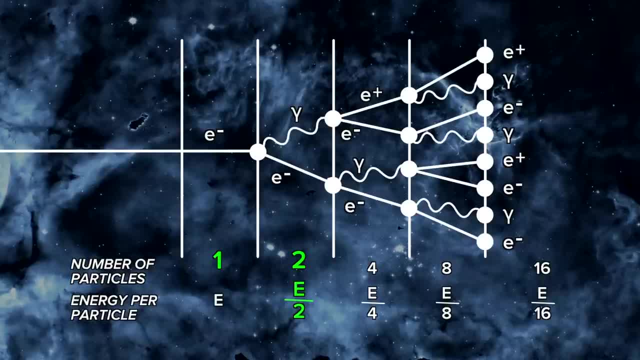 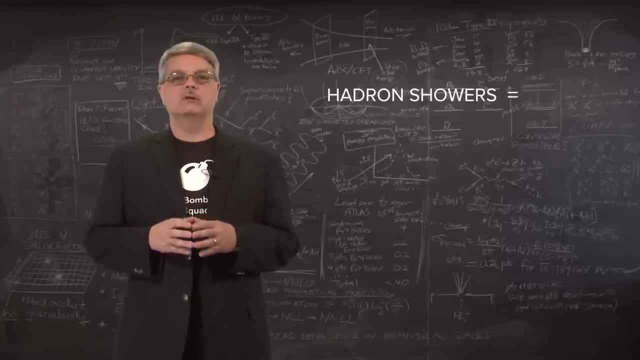 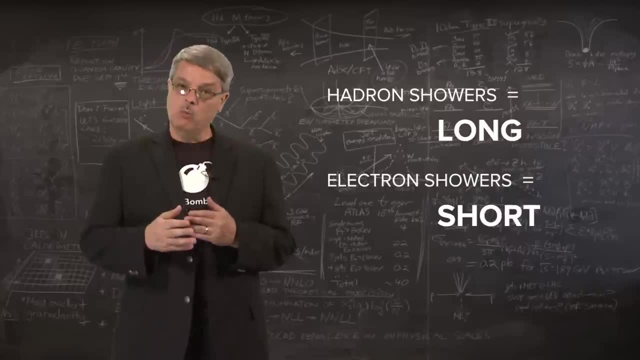 the energy of the first particle. We scientists call this phenomenon a particle shower. Hadron-initiated showers are similar and occur over longer distances. Electron and photon-induced showers can result in over-, Wrestleyr and wave motion, which we don't. showers are faster and develop more quickly. Thus a hadron shower penetrates more deeply. 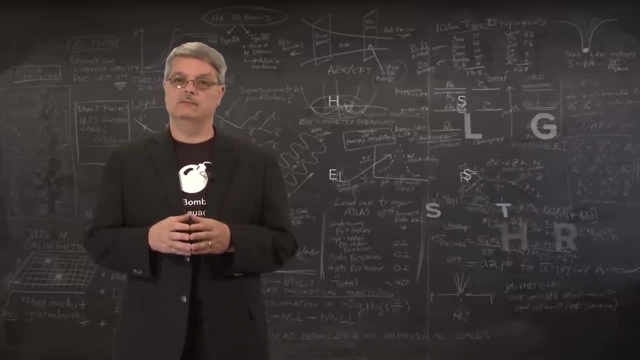 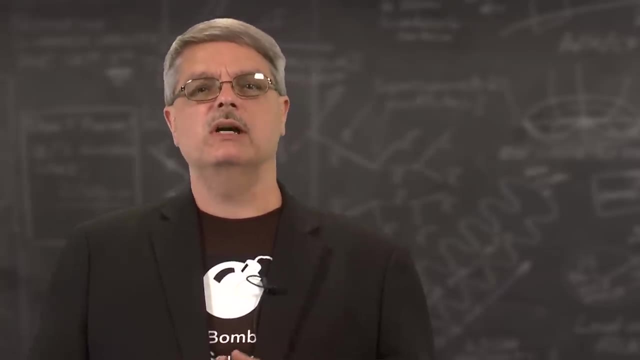 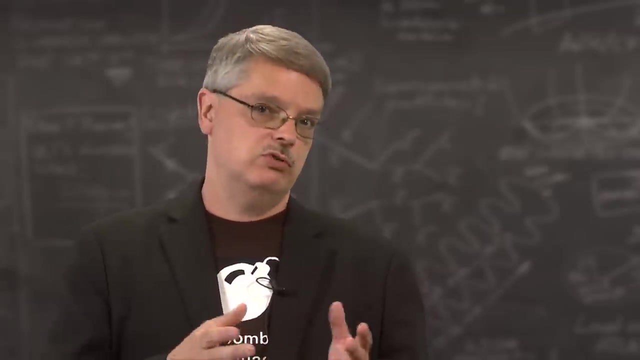 into the detector than one from an electron or a photon. There are many other ways in which particles can interact with matter that scientists can exploit, But just using the two kinds of showering and the atomic shaking of ionization we can see the basic idea of how most particle detectors work using just two components. 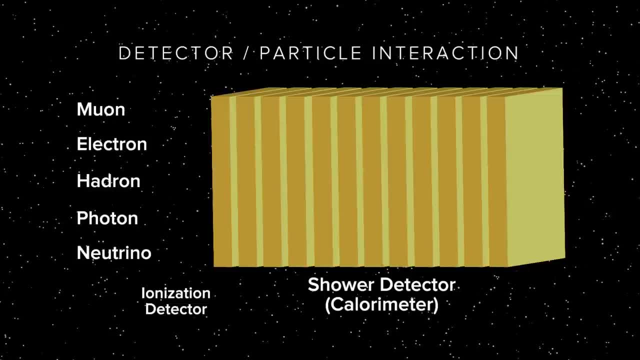 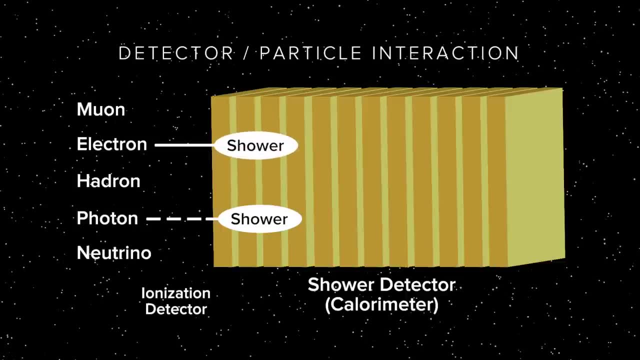 This table shows us how the different particles interact in matter. Photons don't ionize, but make short showers. Electrons both ionize and make short showers. Neutral hadrons don't ionize and make long showers, while the charged ones both ionize and make long showers. Muons. 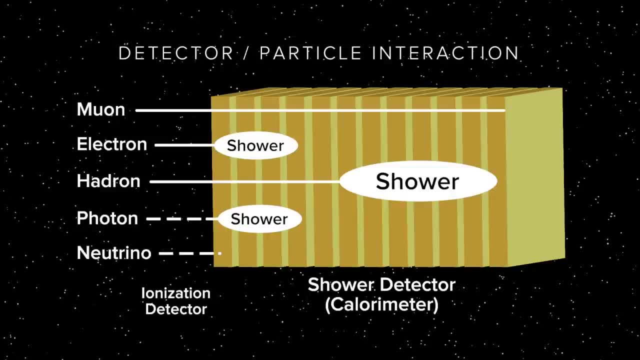 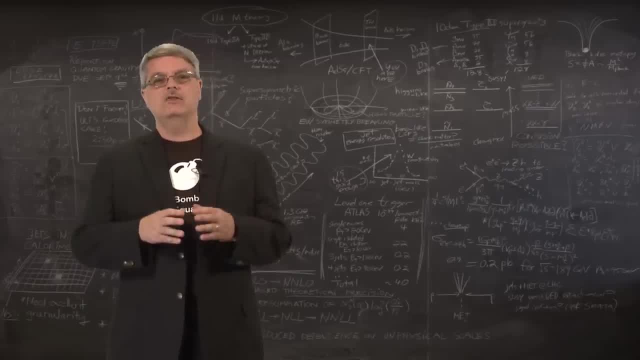 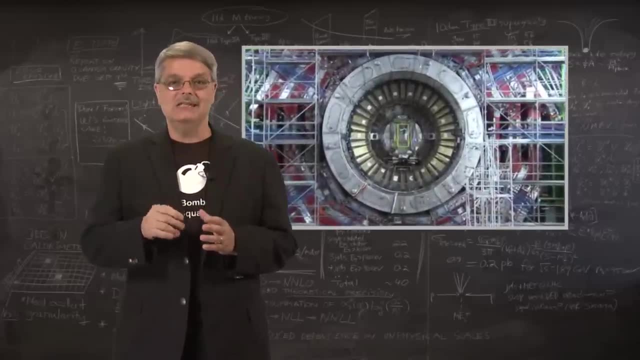 ionize but don't make showers. And neutrinos neither ionize nor shower. So we see that even though we can't directly observe particles leaving the detector, they the collision. we can carefully design a detector that surrounds the collision and see how the 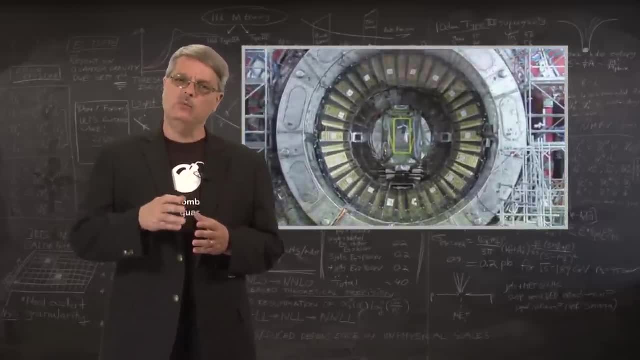 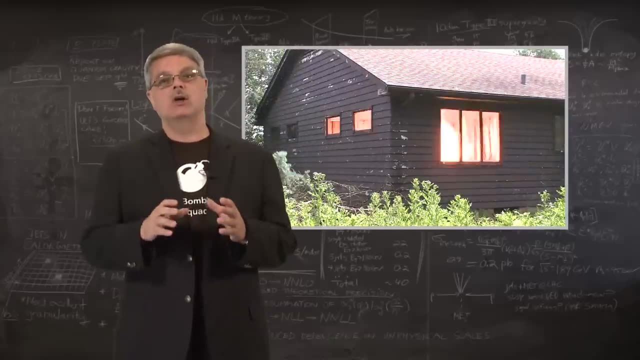 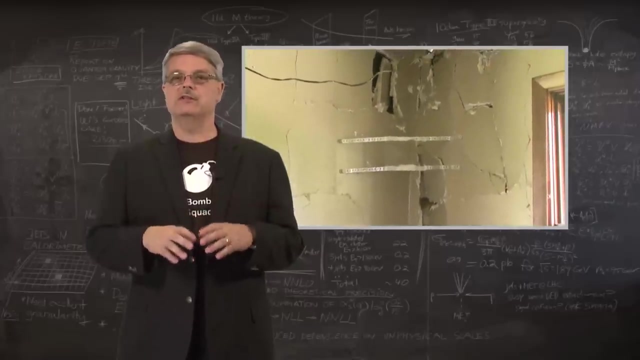 particles interact in the detector. From that we can infer which particles left the collision, and then, finally, we can work our way backwards to understand what physical process caused what we saw in our equipment. In essence, the same thinking whereby the bomb squad investigator can figure out the 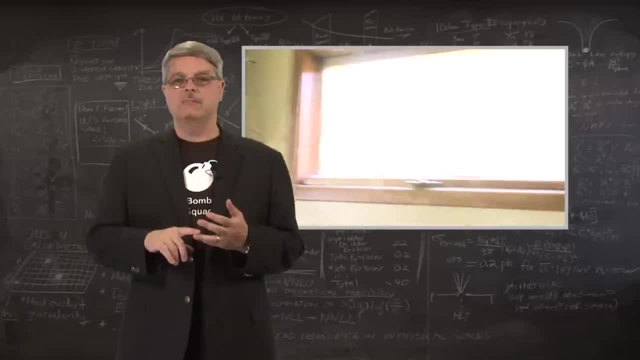 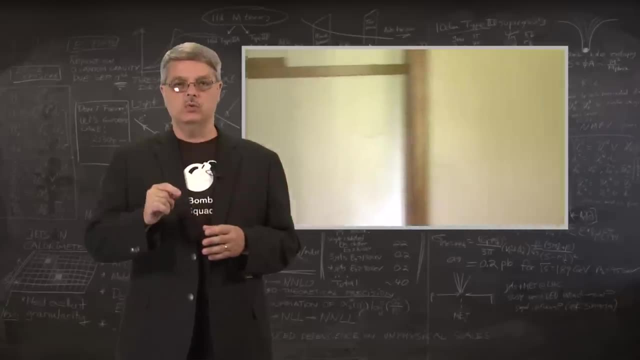 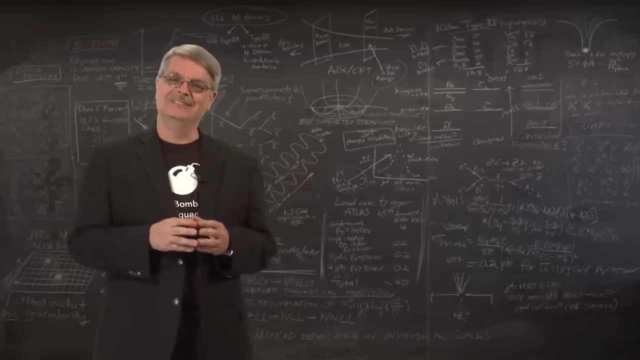 type of explosion, by looking for scorch marks, the depth of penetration of shrapnel, and walls returned and damaged furniture and so forth, is what we particle physicists do to reconstruct our collisions. You know, subatomic bomb squad investigators has a really nice ring to it, don't you think?